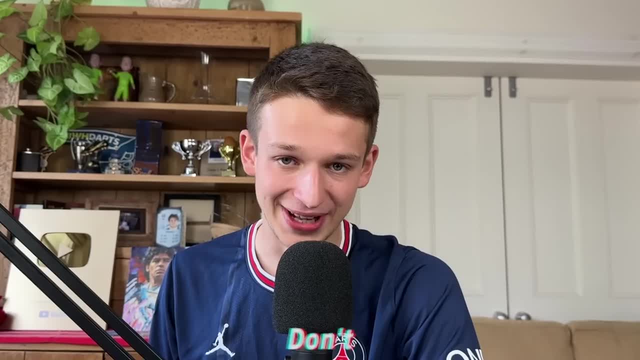 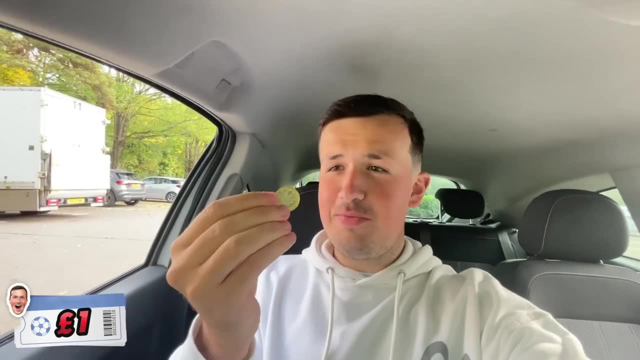 One thing, Theo. I live three hours away, pal. How am I going to get there? I don't care. Teleport, mate. Water raft- No, Enjoy, mate. Here's your £1 coin. Whoa Foggo's mugged me off here. 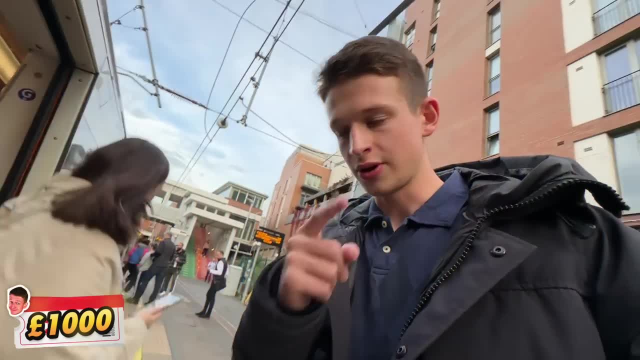 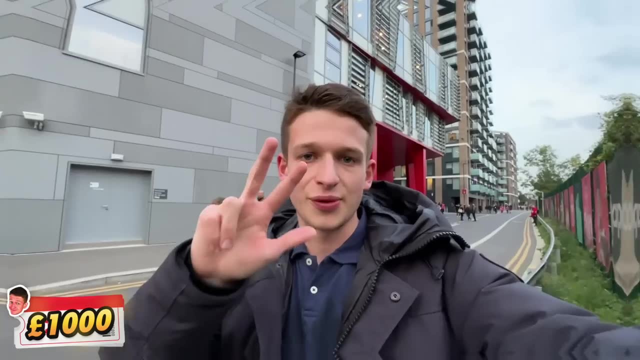 Now I've got to drive three hours to Coventry. You're having me on, So Theo has to travel down the road and Josh has got to travel for three hours. How is that fair? Three hours till kick-off. We have made it to the Brentford Community Stadium. 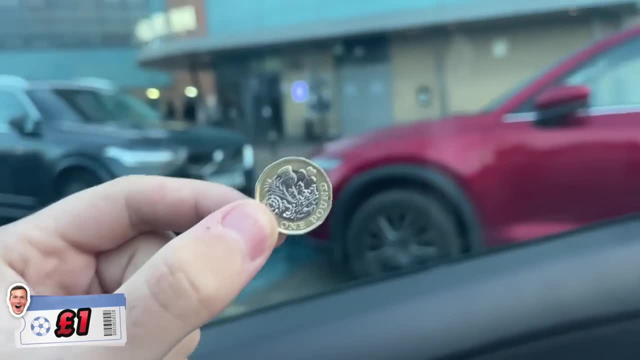 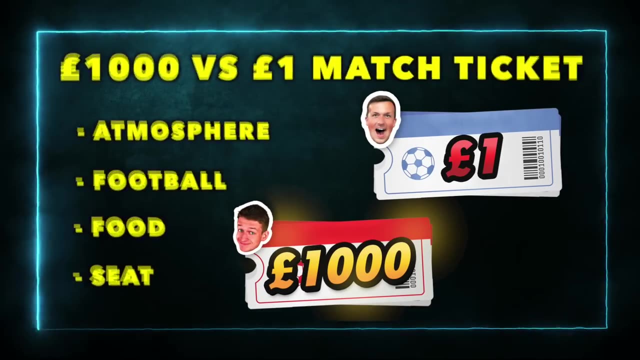 I've been travelling for the last three hours with this £1 coin to watch some football inside that stadium, Whilst Theo is just down the road at Brentford. How unfair is that? by the way, Those two mugs are going to compare the intensity of the atmosphere, the quality of the football, the tastiness of the scran and the comfort of the seats. 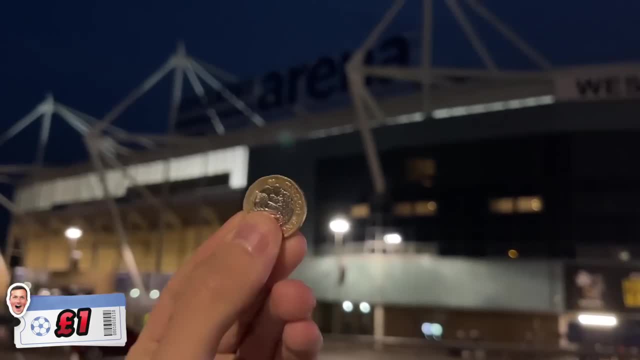 Hello Jono. How are we doing? Good to see you. What should we expect today? I've got to go get my ticket for £1.. I want you to have the VIP experience, so we are going to go into the Orchard Lounge. 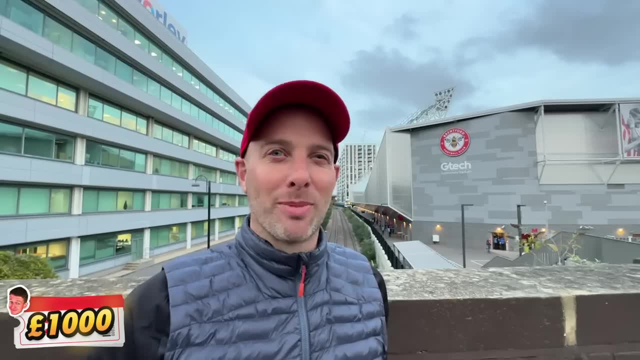 We're going to have the Michelin-starred Indian food. Wow, We're going to have the chat. We'll be in a nice relaxed environment. Yeah, smashing Should be an epic night. So let's get the guys into the ground. 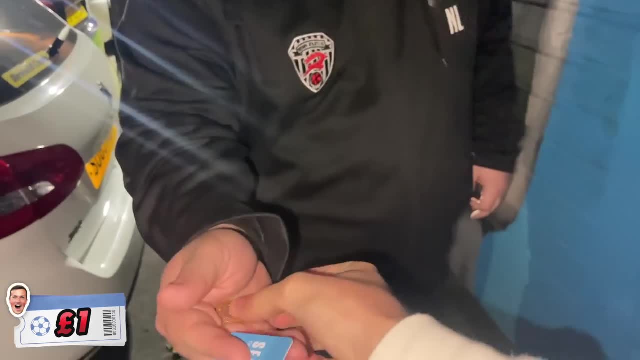 Wait a minute. Who's taking my job? Neil, here's your pounds. There's your ticket. Josh, Here's your ticket. Come on. So this is the personal service that you get. There we go. That's what we love. 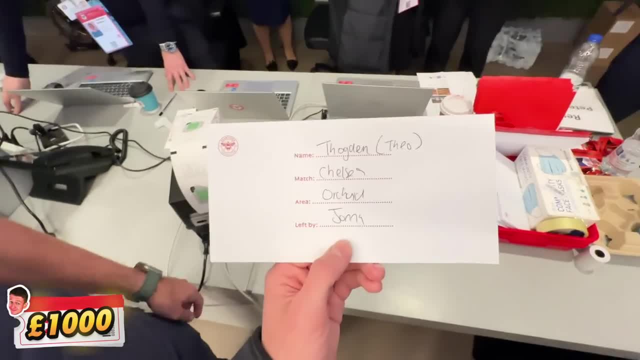 Thank you. They look after you here In my name. Just make sure you get all sorts. Oh perfect, There we go. Thank you very much. You're going to need that. Can't miss out on these two. Thank you very much. 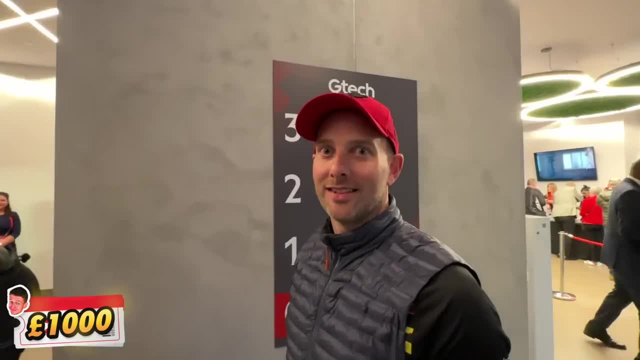 Cheers mate. We've been given a little lanyard here saying Brentford versus Chelsea. You've got a lift at a football stadium. That is unbelievable, It's very exciting. You think a lift at a football ground is exciting? 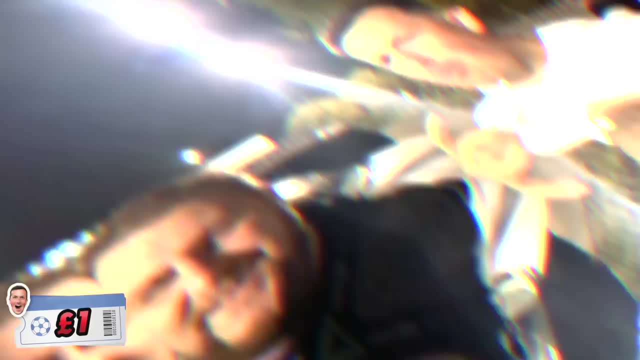 Give your head a wobble, lad. That is a proper experience. Josh has sorted it out. What is the experience going to be like for £1?? And this ticket is insane Value for money. How's the atmosphere going to be? 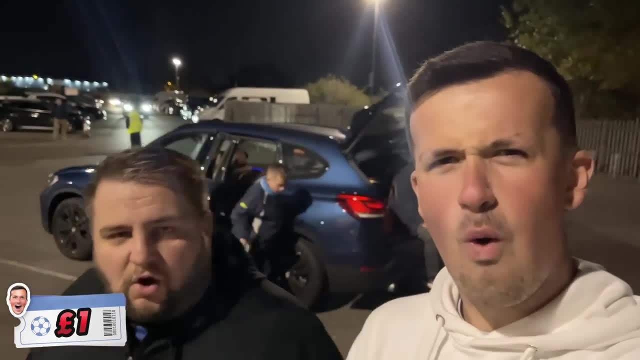 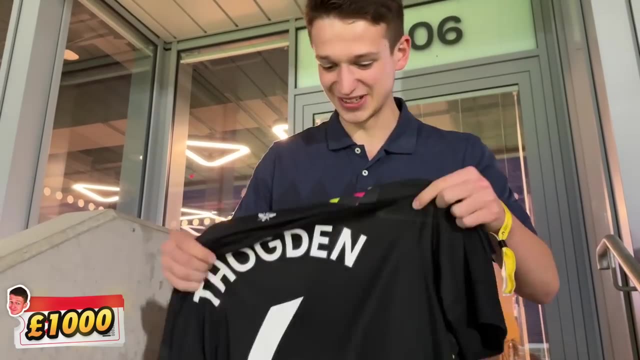 The atmosphere is going to be rocking. We've got a big crowd in here tonight. Here it is, Let's head inside. We've made it to the G-Tech Community Stadium. We've got our little care package. I've got a Brentford shirt. 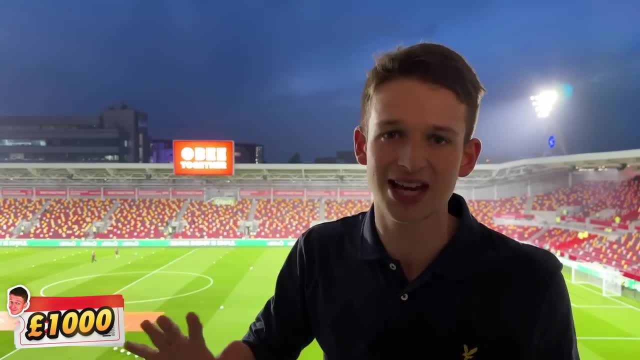 Wait a minute, doggy, You can't wear that. You're a Bolton fan. The stadium: it's a solid 8 out of 10.. It's one of the newest in the Premier League, So I'm excited. Let's give it a go. 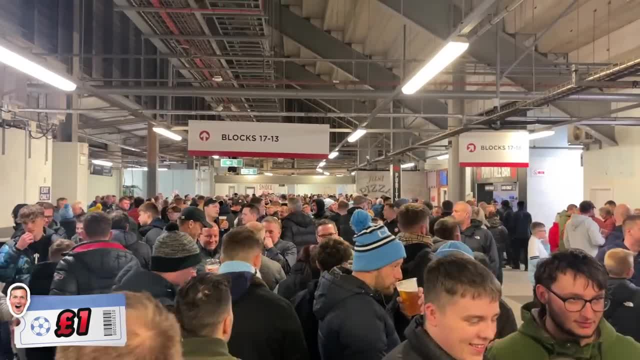 Let's go over to Josh. Has he made it to the stadium yet? Theo is not going to be experiencing something like this in a corn course. I've already spent £1.. I've already spent £1 on the ticket. I can't get any food or drink. 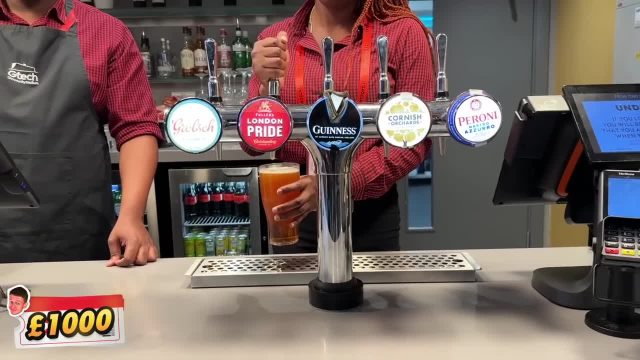 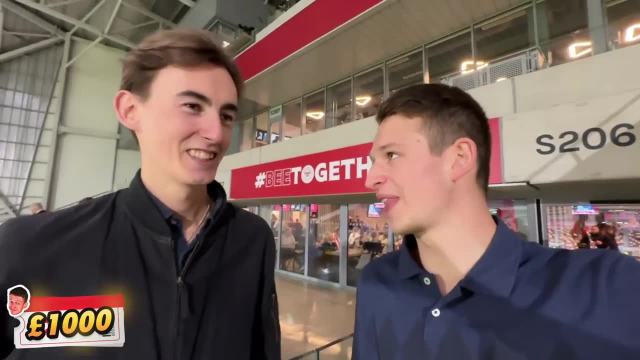 And Theo's got unlimited bar and everything. We're inside the lounge. What's your thoughts on the ground? I mean beautiful ground. I've sent Josh to Coventry against Sheffield United- £1 ticket. What do you think about that? 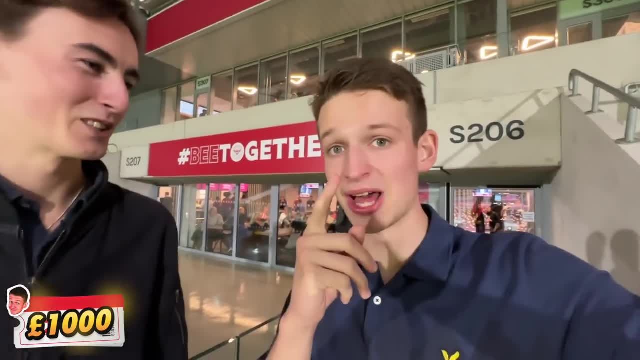 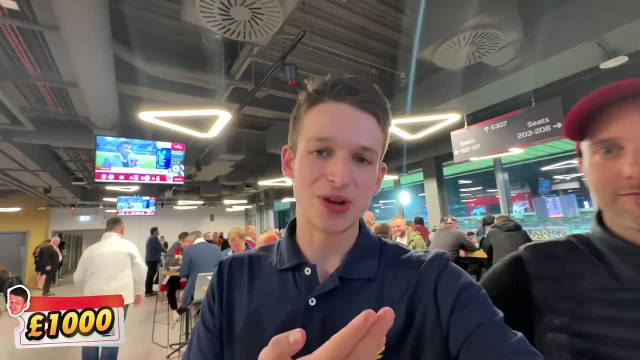 They did So the Coventry fans might be loving it. So to watch Coventry it cost me £1.. What do I expect today by watching Coventry? It might be bottom of the league This season. not a lot Inside the Orchard Lounge. 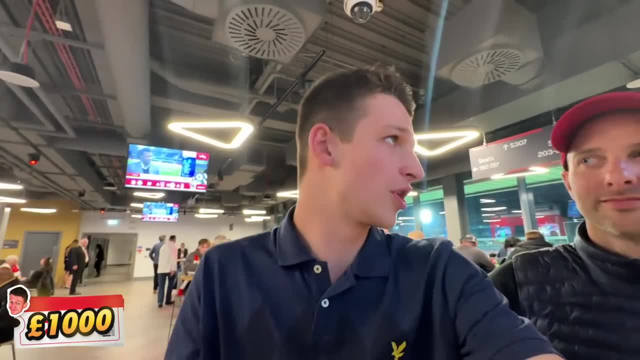 We've got to do a little attempt at the food and the drink. Give it a review and compare it to Josh Over in Coventry. Over in Coventry, Roasted aubergine chicken tikka masala. Should we give it a go? 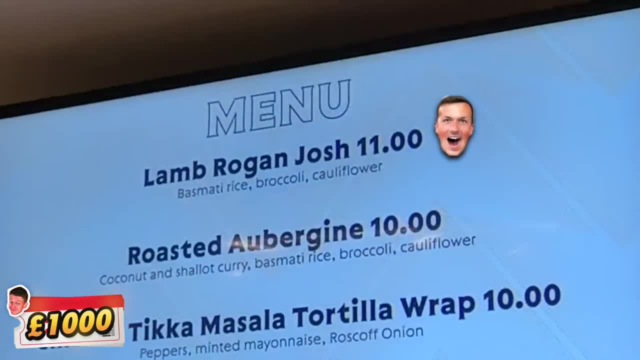 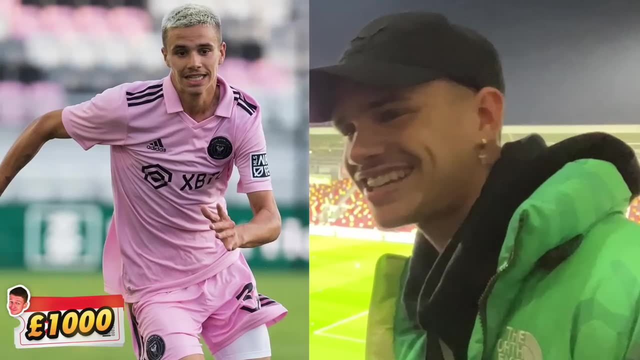 I think there's going to be a lot of Josh eating tonight. We might have to beat Josh Chilling out at the G-Tech with Brentford's top talents. Wait a minute. Isn't that David Beckham's lounge? A place for Inter Miami? 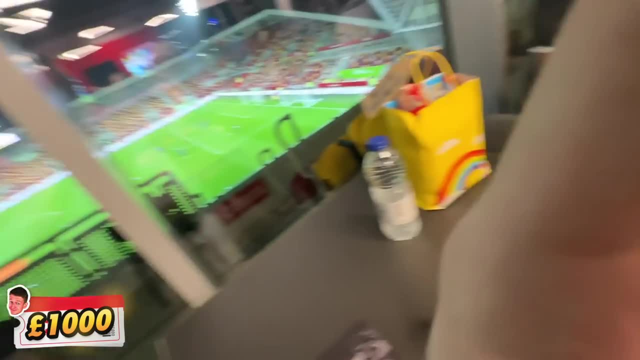 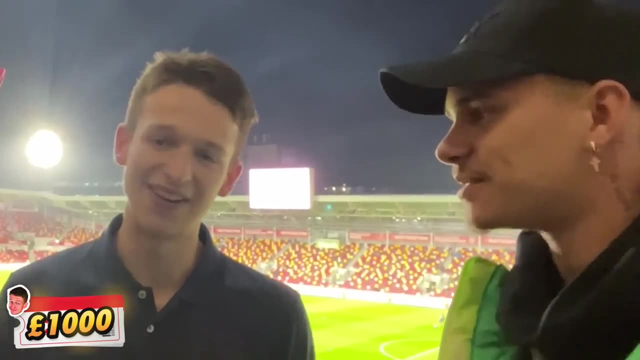 We are living the experience, the luxury life. What do you think about these seats? Is it worth the money? Yeah, 100%. It's the best sitting money can buy you: YouTube's millions of subscribers. YouTube man, Oh, it's too tight. 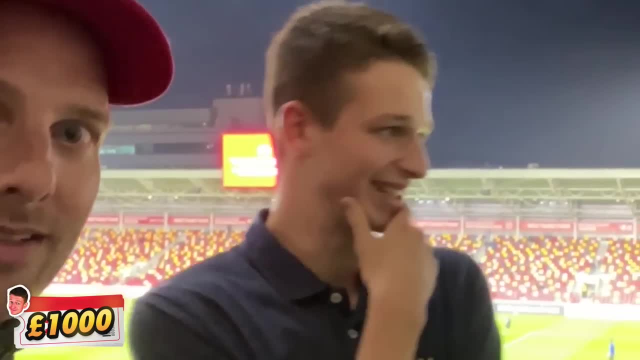 Yeah, yeah, It's got a channel as well. It's got a 3-0 Brentford's. When do you think Brentford will finish this year? I think they can go for a little European run. Yeah, Yeah, all right. 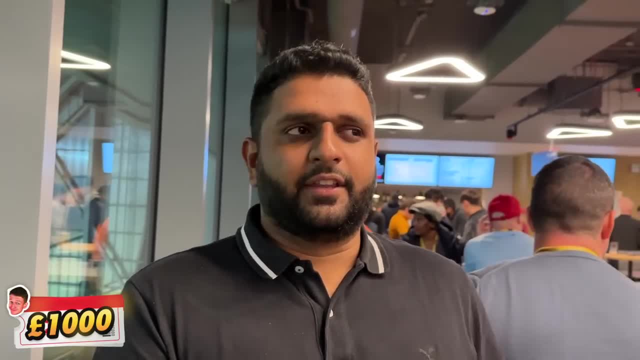 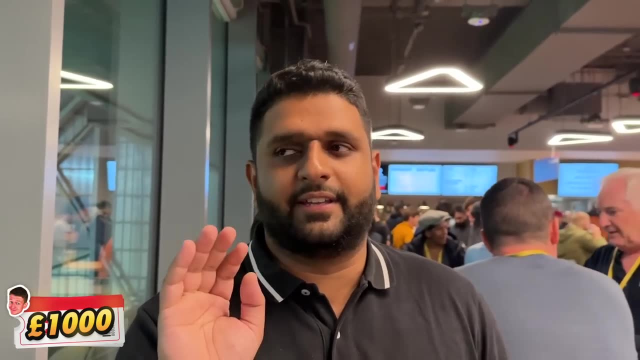 For a pound. it'll do, But is the atmosphere still good? Yeah, You'll come out and you'll hear Hey Judah, just before kick-off. Okay, And that's the best experience you'll ever witness in your life. Atmosphere-wise. 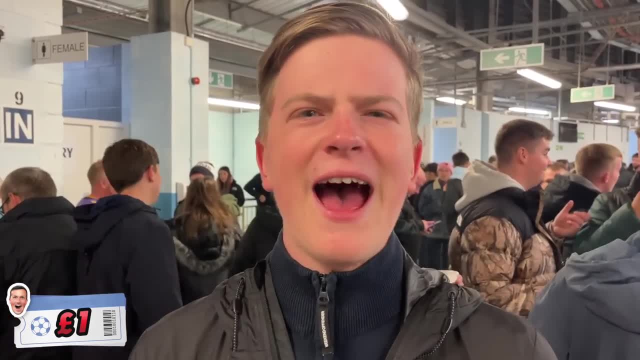 That'll be good. It'll be good either way. For a quid it must be all right for our atmosphere. Yeah, of course it will. Yeah, Koresh Moroni personal review here. That's a solid 7.1.. 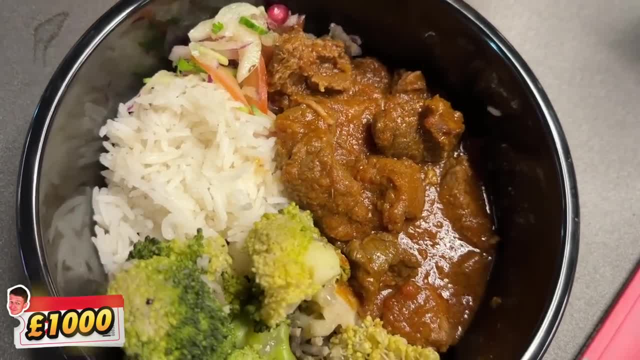 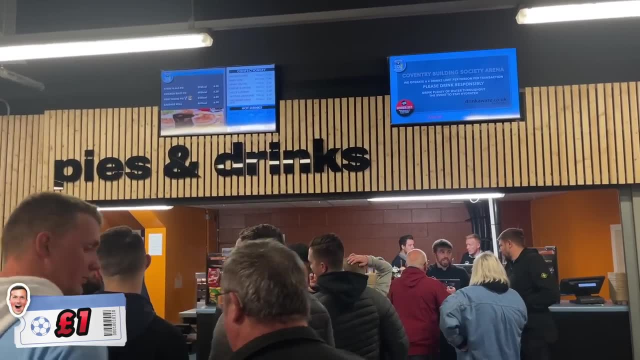 A lamb, rogan, Josh- And I know Josh will not be having What Such good food. This one pound is no longer going to be one pound because I'm hungry. I'm sorry, Theo, I'm going to get some food. 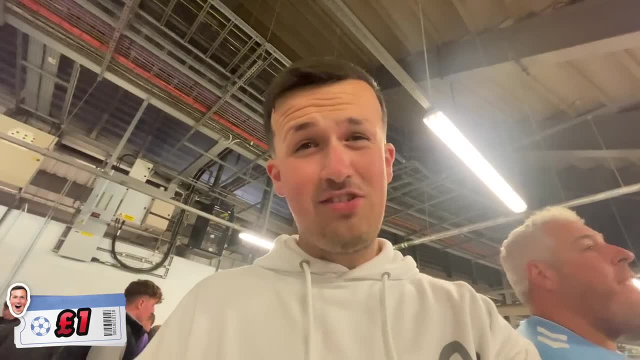 This man can't let me starve. I've got to get some food and a pie it is, And I bet he's got a pie for free or something. Where have I said Josh? I've said him where We're chatting to Coventry. 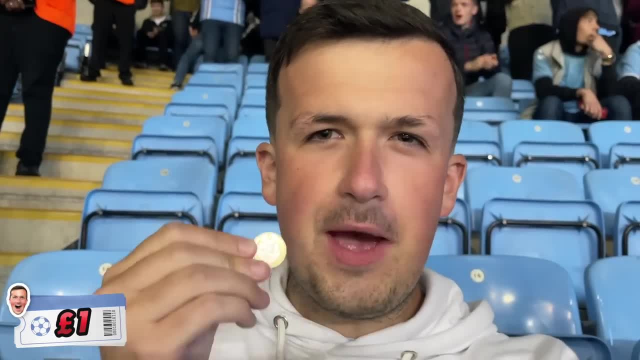 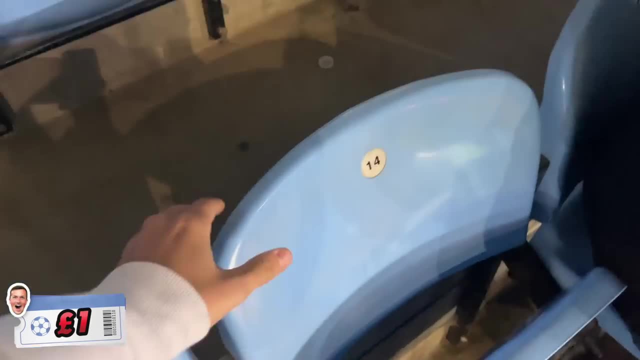 Yeah, Oh, love the dad joke, mate. Does Theo have an atmosphere pre-match like that? A little seat review. Take a look at this padded seat. Josh doesn't have that, And here's my seat today: Plastic seat, And I bet Theo is in a nice leather seat right now. 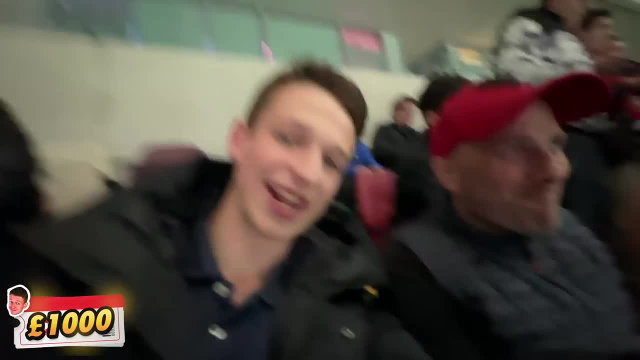 Josh liked the seats as well. actually He was quite interested in that. He will not be getting that in Coventry. He will be on a plastic seat in the cold. I'm freezing. I bet he's warm in a nice environment in his hospitality. 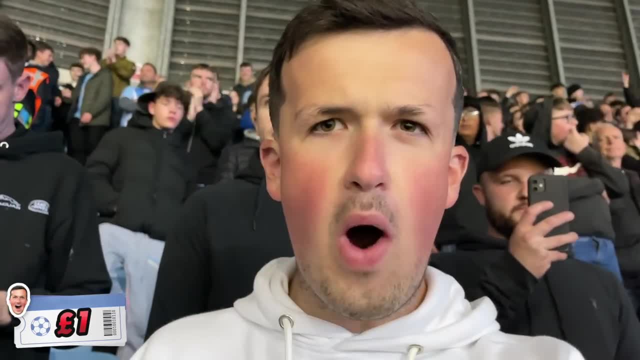 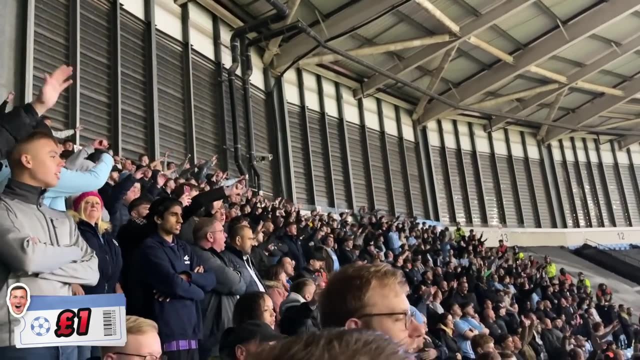 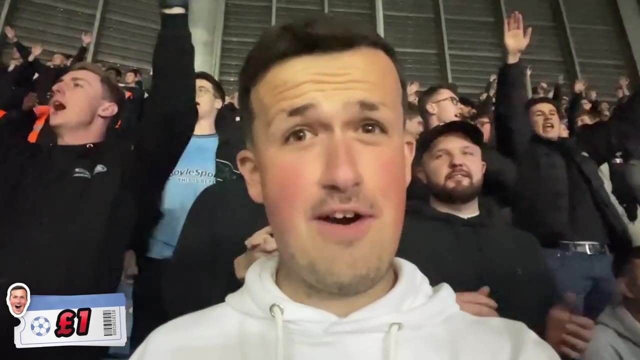 The last five games for Coventry have either been 0-0 or 1-0.. You know, tonight the football side It's going to be minimal goals. Coventry out this minute. Give them credit. Give them credit. They're the best in the NFL. 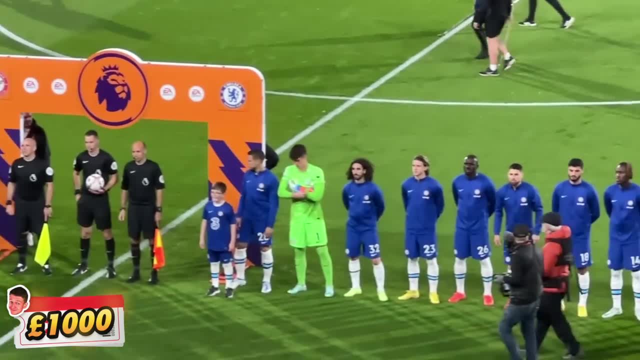 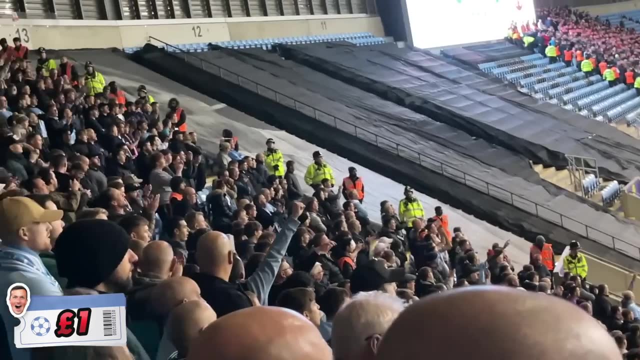 Brentford and Chelsea West London. Which colour will it be after 90 minutes of football? Football for a pound. Welcome Coventry versus Gefford United. We've got a big swing on our side. Get the day up. So far it's a 0-0.. 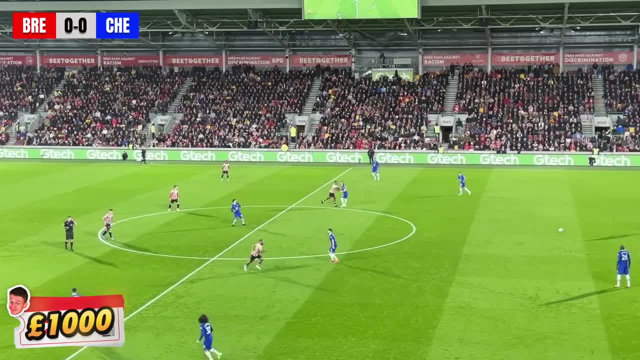 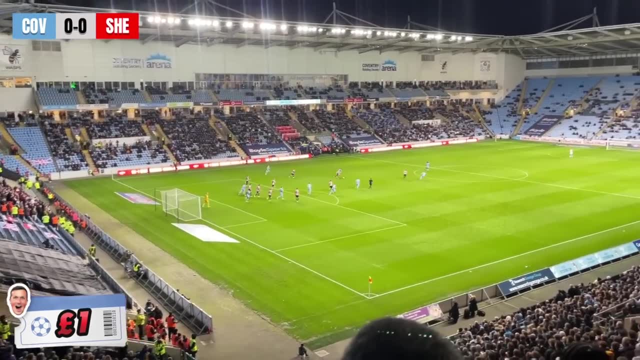 It's cold And it's a good atmosphere though. So over in Brentford, the El Chisico has kicked off, And meanwhile over in Coventry it's the start of the El Covo. Brentford are all over Chelsea. 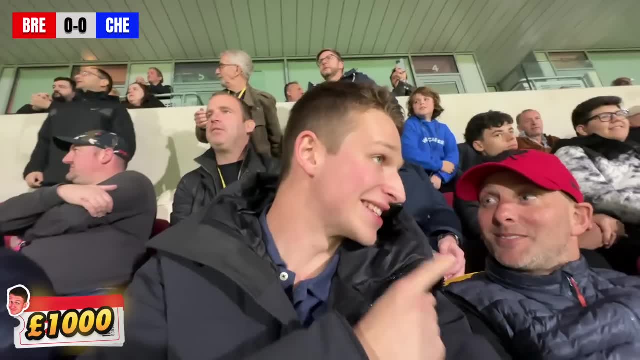 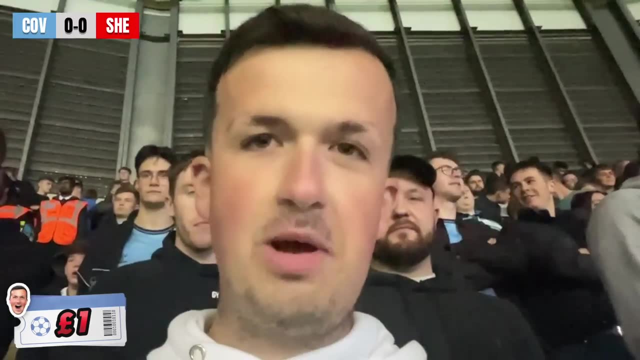 What's going on? They are playing their best football, living their best lives. We need to find out what's going on in Coventry. Oh no Guys, This is going to be the highlight. I bet that explains the football we're watching today. for a pound. 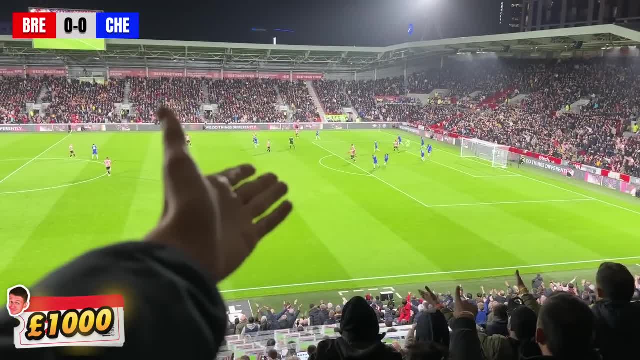 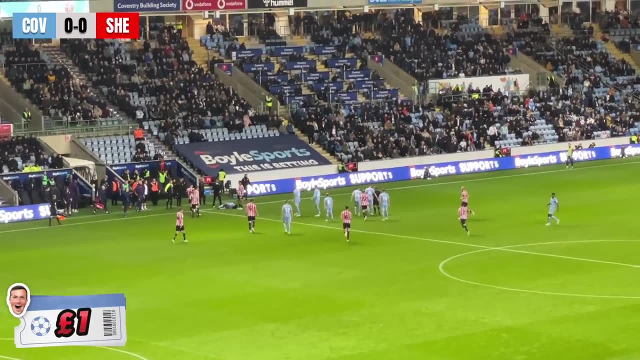 Rico Henry, that's a pen. That's good. That'll be a pen Ref. where's VAR? Yeah, I know, Go to it. All the action here at the T-Tank Proper EFL action. I haven't got a clue what's going on. 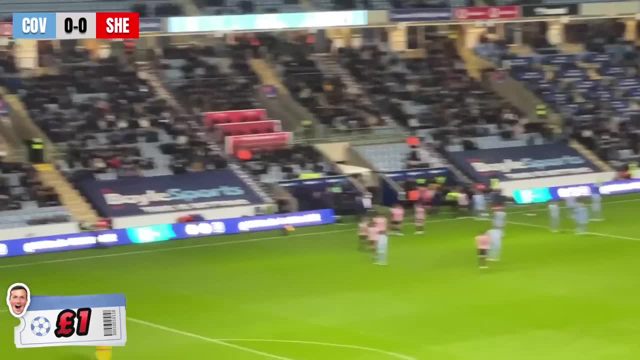 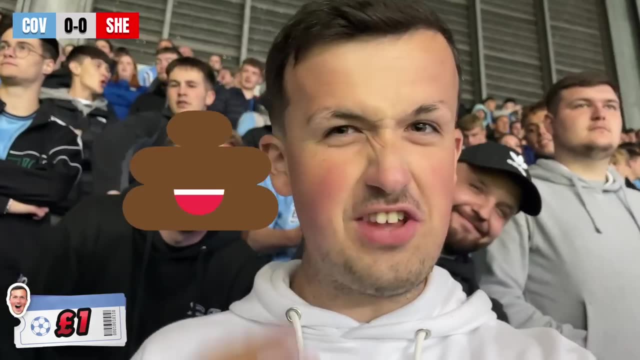 It's all kicking off. It's all you love to see. Oh, fuck off. You're my best referee. You're my best referee Referees- they stink. So with our seat we get a free magazine. 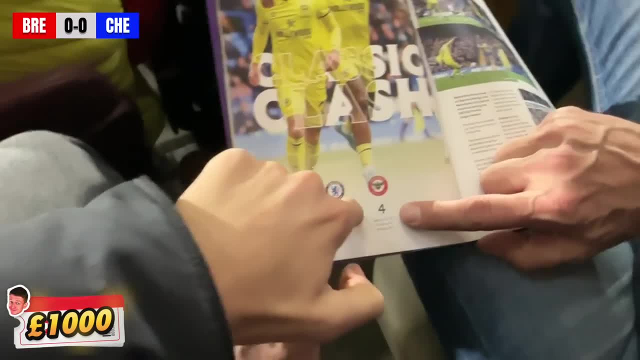 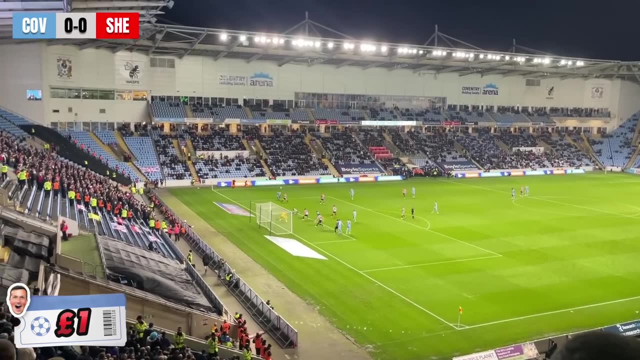 We do, we do, And I'm just enjoying the score. last time they played together. Will that happen again? Football has not paid off yet. Let's see what's going on in the mid-law. On half-time There's a corner ball, though. 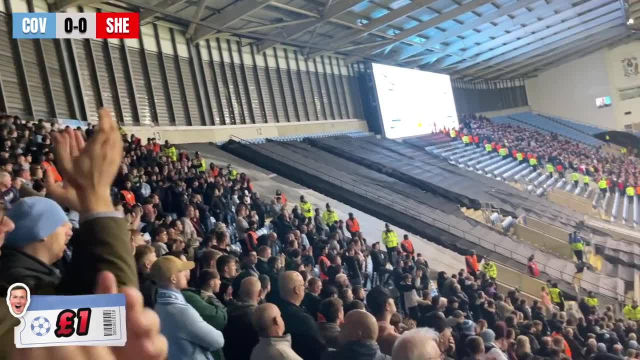 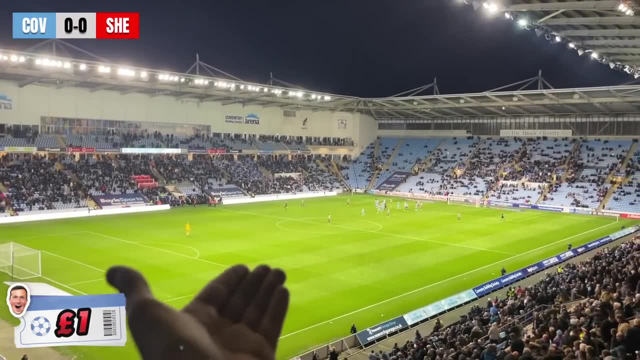 Oh yeah, Come on, And it's half-time. Half-time, Oh, and a boozer for the referee, because they're worth a quid. This game's been pretty boring, I'm not going to lie. It's been very comfortable. 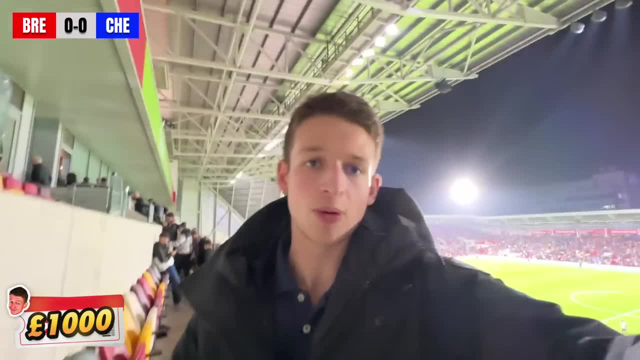 It's not like I'm at the cinema. you know The expensive tickets. it's got all the qualities. We're about to go into the warmth, We're having a beer. we're having a pint Free pie, free beer. 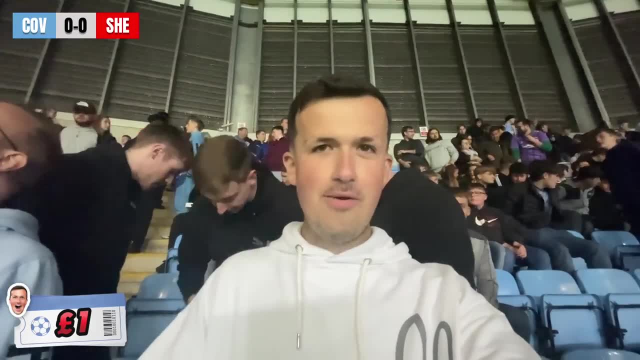 That'll be good, That'll be nice, That'll be great. Thank you, beer, for sending me 0-0.. Absolutely nothing's happened that first half, But hey, I bet you're enjoying a nice warm seat. levered seat. 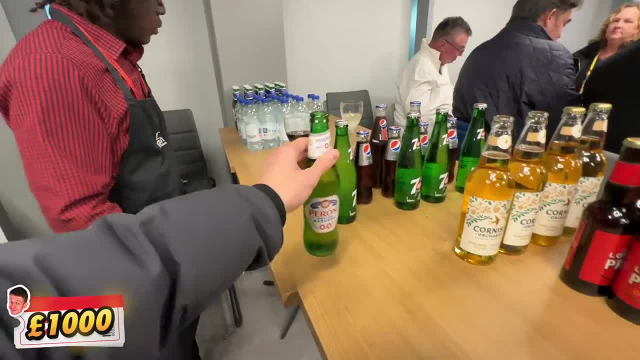 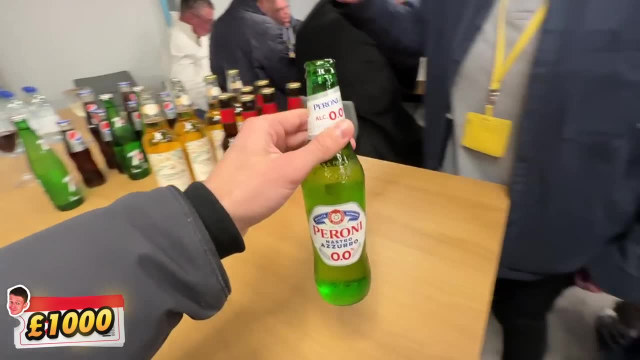 Absolutely beautiful And you're making me watch this. Thanks, mate. Zero percent, Hold on. No, son of mine drinks a zero percent beer. Come on, lad. Oh, that is better, mate. Well done. Please be mugged off. 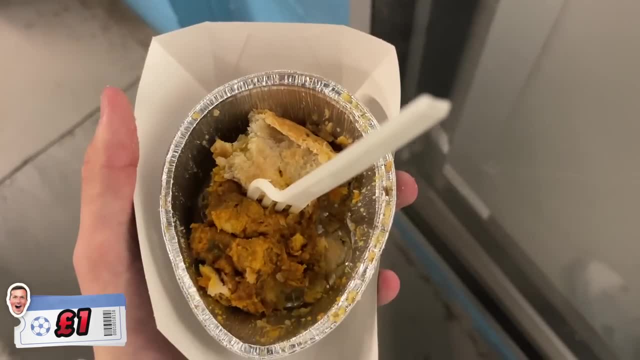 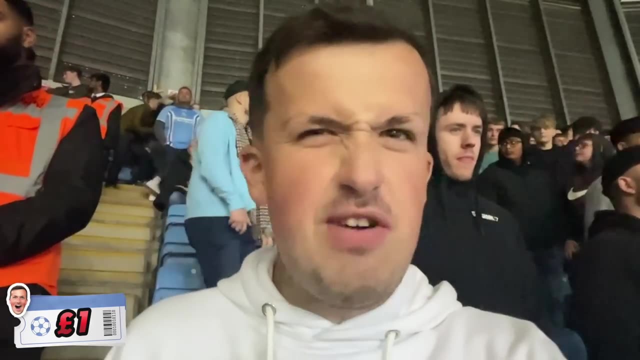 But no, we got ourselves a little hot again. I've had my cry- which was very, very decent, I must admit- Over the £1 budget. I'm so sorry, I'm hungry, I can't help it. But Theo, that half-time, did he have any refreshments? 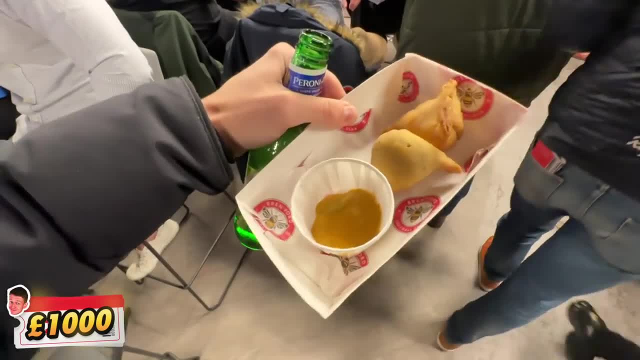 So here's what you get in the Orchard Lounge at half-time: All free Samosas today, mixed up the menu and a Peroni. I like that. However, the steak and ale pies they had at Griffin Park Director's Box were unbelievable. 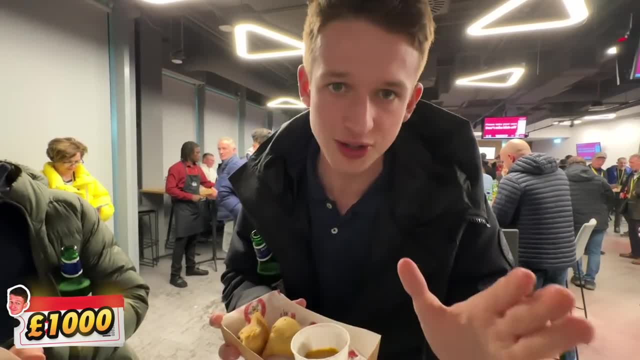 And apparently they usually offer pies at half-time. So, gutter, not to try that. What's your experience in the lounge? Because I've sent Josh to a £1 football match today. I think it's great. Yeah, And we're back. 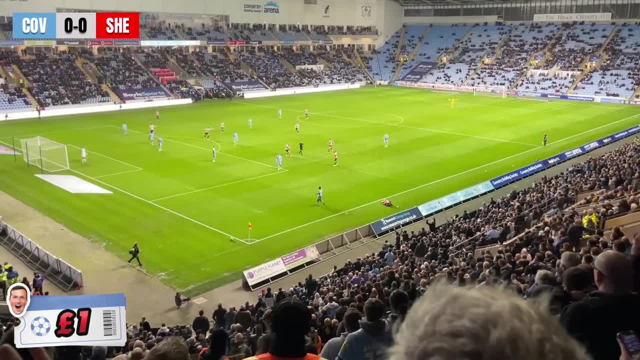 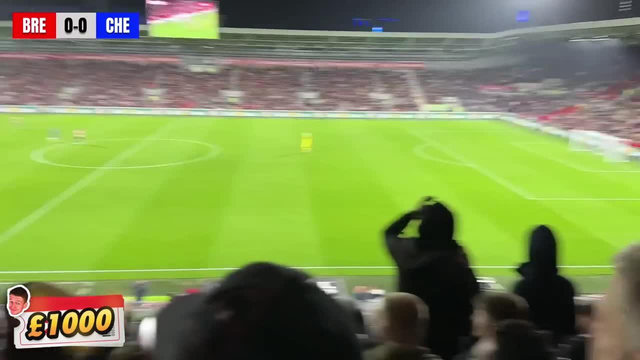 Second half, Here we go, It's gone, It's gone. There must be a second yellow. It's gone. That's a second yellow. The officials are so bad. Kepa saves. Kepa saves Energy's building. 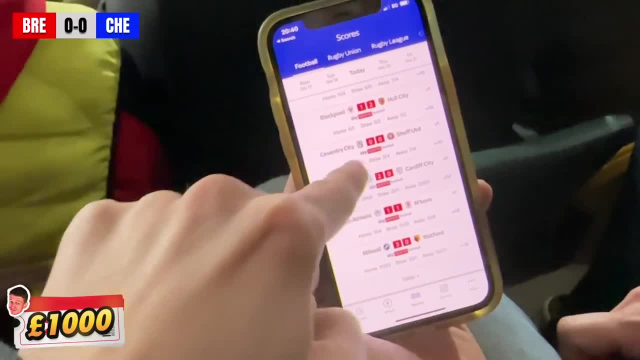 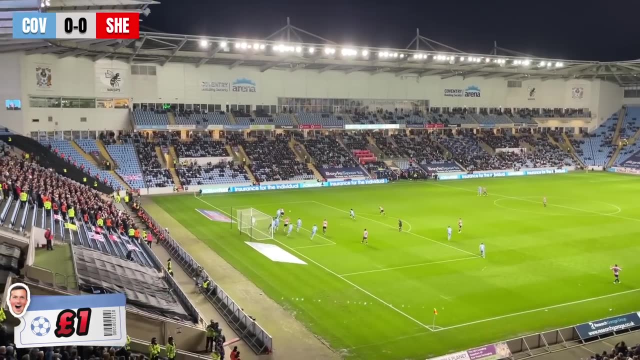 Yeah, It's on a knife edge. We've just found out it's nil-nil at half-time in Coventry, Sheffield United. What if we watch 180 minutes of football with zero goals? This will be the worst video ever. Oh, Oh my. 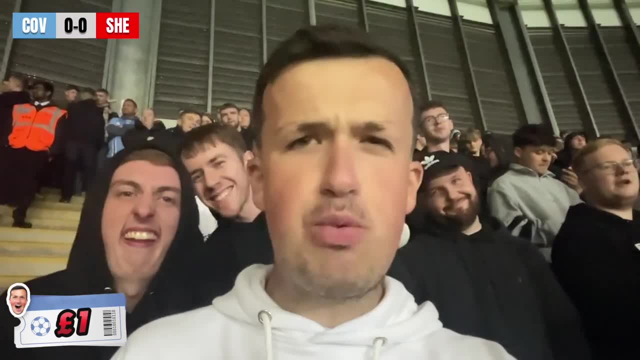 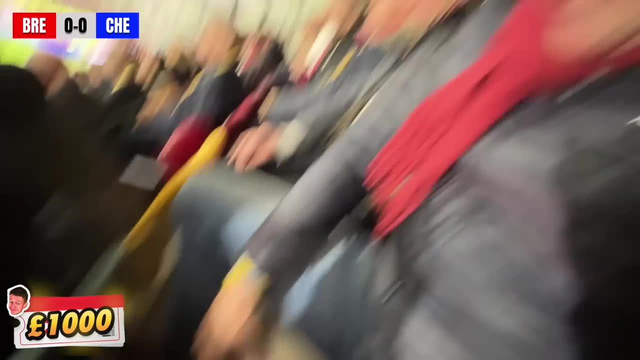 Look at the state of that mug. I've seen this story before that starts with Mbwemo. Oh my God, Oh nil-nil-nil. Look at the plush Padded seat review. These are seriously plush seats. Yeah, quality. 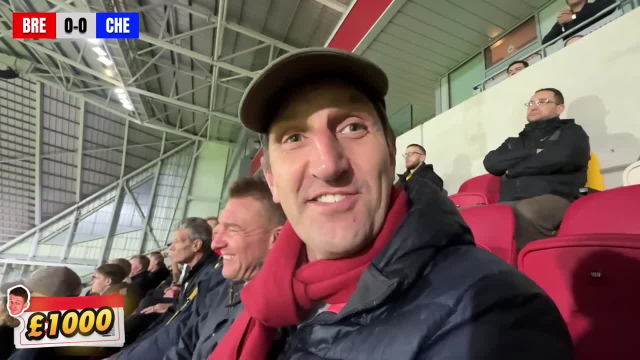 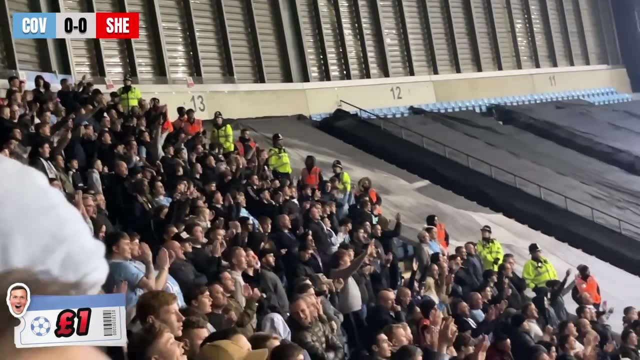 There is- you know, this is VIP service- the Van der Plaar seats. Doggy, get that man a prawn sandwich. The only cost a million. The great thing is what's a million, Gustavo? Hey, hey, hey. 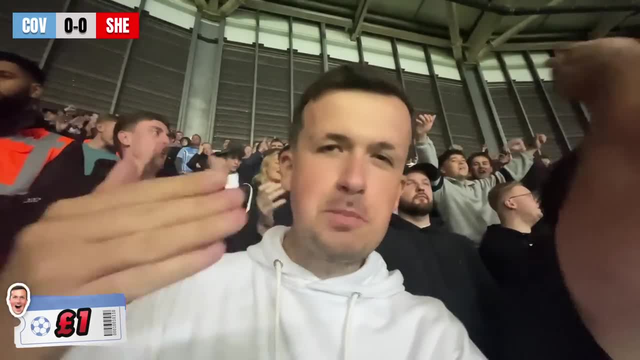 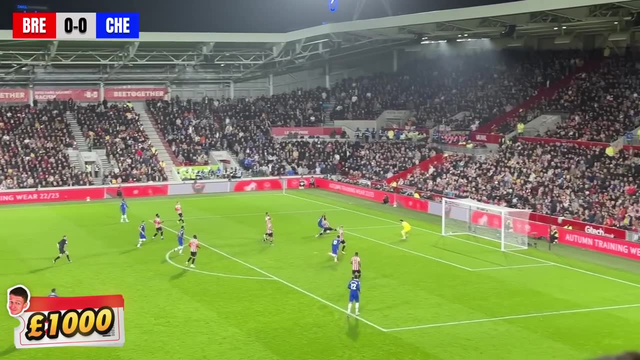 You're not getting this video. You're not getting this video. No, I'm not. It's not your hospitality mate. Listen to this: A nil-nil in the championship. You don't get this in the front mate. It's good football reinstalling. 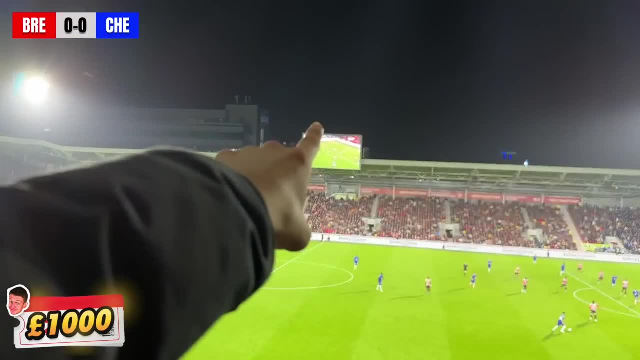 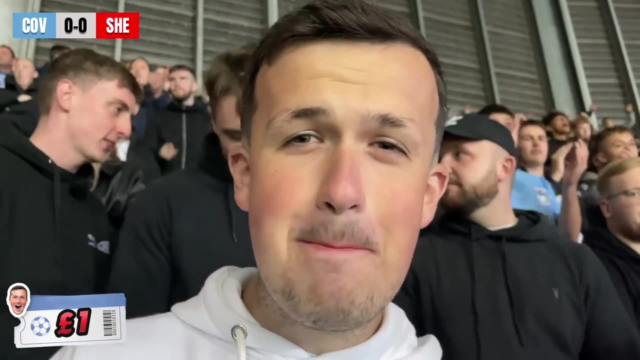 That's called it. Still nil-nil in Coventry, Sheffield United. Still nil-nil in Brentford. Won't somebody please score a goal somewhere? You talk about the football. It is absolutely diabolical, But hey, the atmosphere is good. 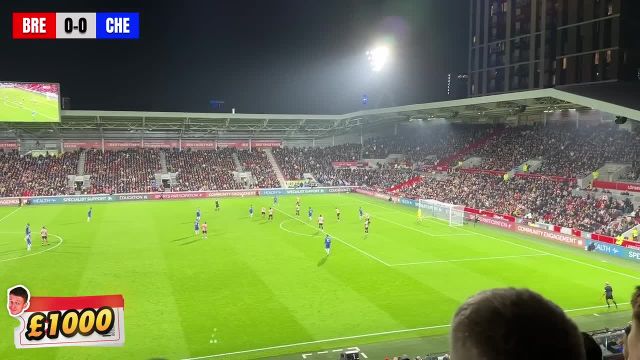 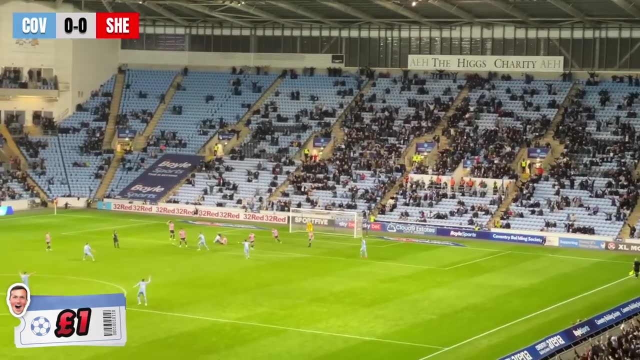 That's all I care about. Pulisic saved Aubameyang predicts it Nothing. He can't take it. It's goal time. Gurkhez, Play it. Oh, Oh Woo. Trust control Four minutes at a time. 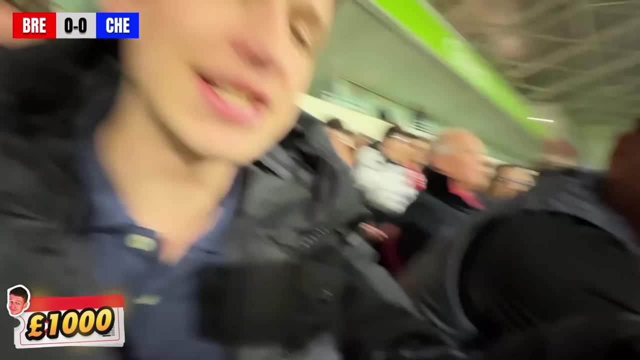 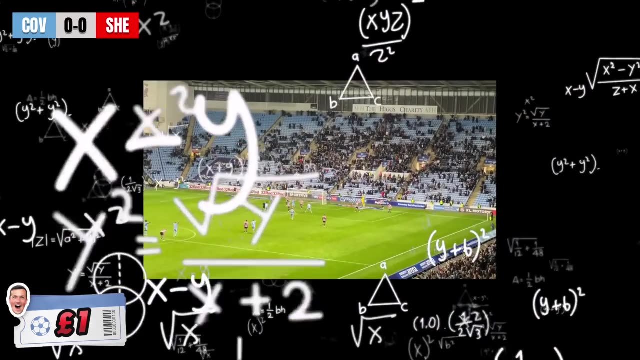 Anything can happen. Oh, what a save, David Raya. David Raya is number one for Spain. He's not De Gea, not Pepto. Oh referee, that's a nailed-on penalty, Don't you know? we're making a video here. 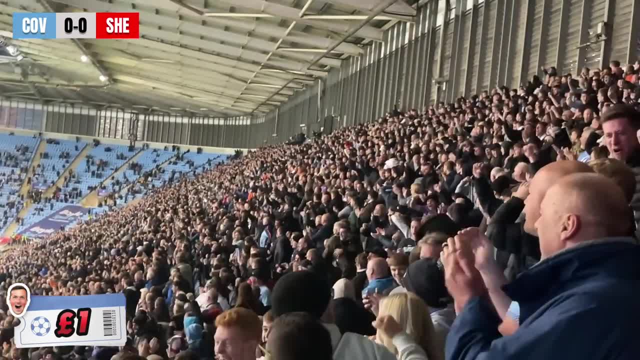 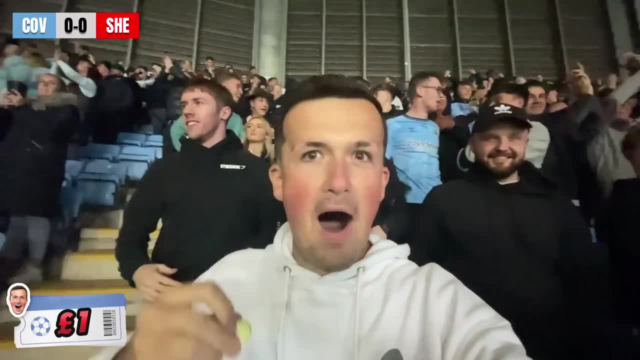 Come on, ref. Point to the spot. Come on, He's given it. He's given it, man. There's a penalty to Coventry. Can they score Four for the Pound City? Come on for Steve Glynis, the ESL. 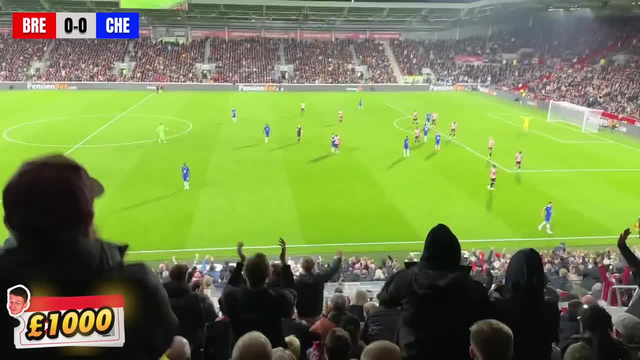 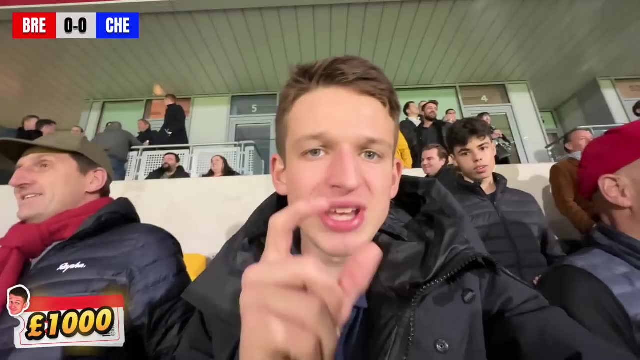 Does Michael score? That is full-time here in Brentford, Played that all day. yeah, I've enjoyed the experience today being within the lounge. Ticket money can't buy. We start at 7.30.. Josh's game is a later kick-off. 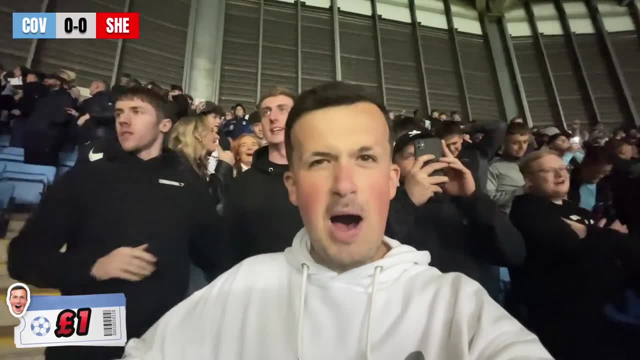 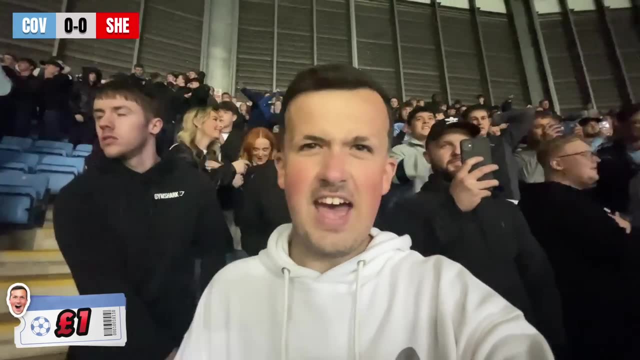 So let's go over to him for the last five minutes. This is the moment in my plastic seat. Move the fans where the limbs, the seams, are. But Theo, he's in hospitality, He's in this, he's in the warm seats. 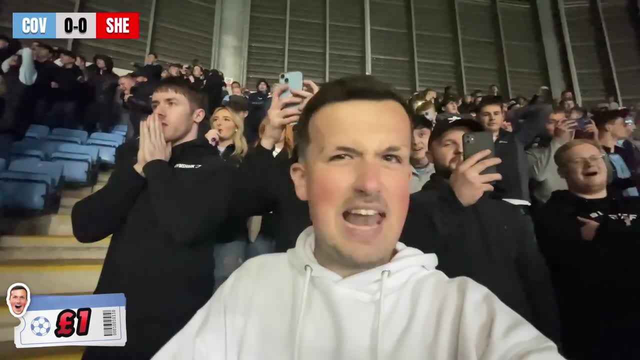 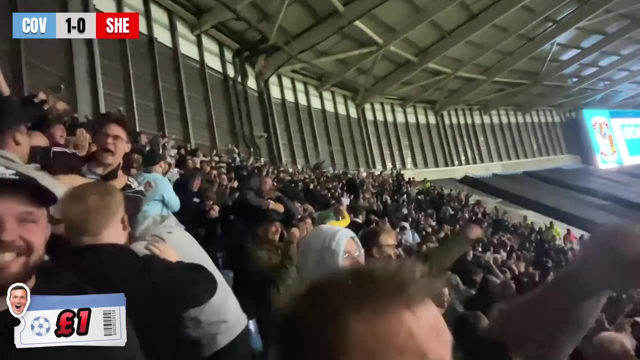 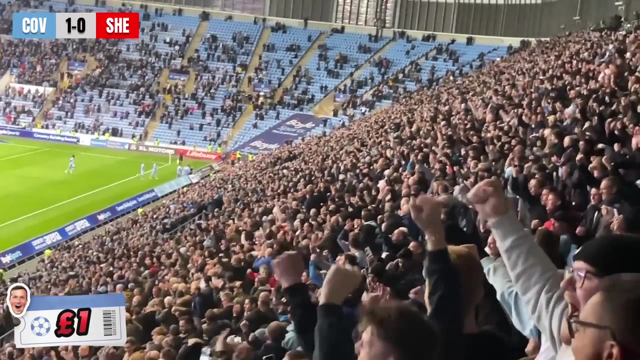 He's in the posh area, But he doesn't get last-minute, late seams like this. does he Last-minute? Yeah, Absolute limbs there at Coventry. What an atmosphere. That just shows you don't have to spend more than a quid to enjoy your football. 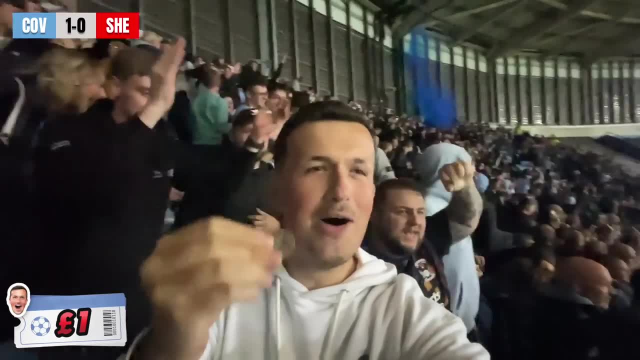 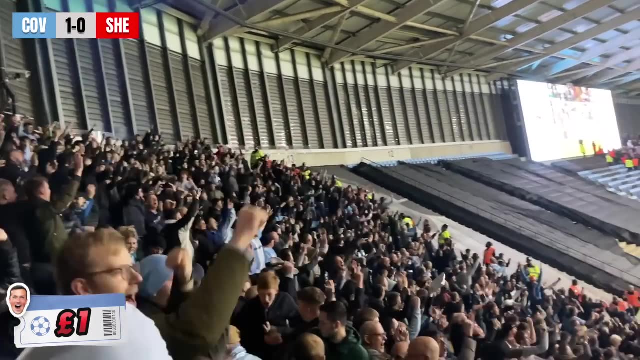 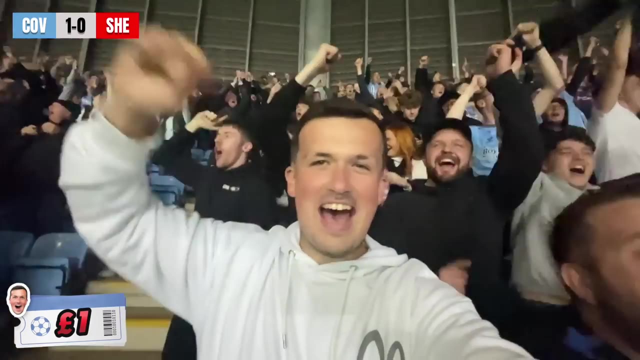 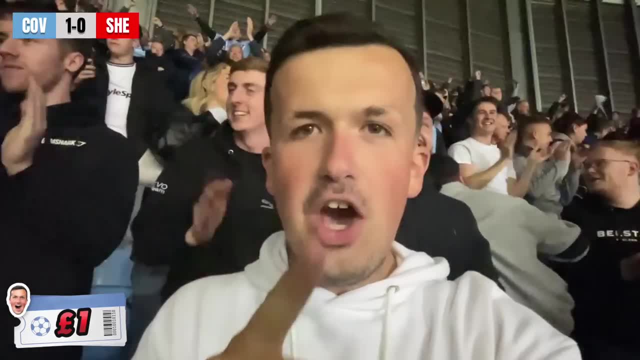 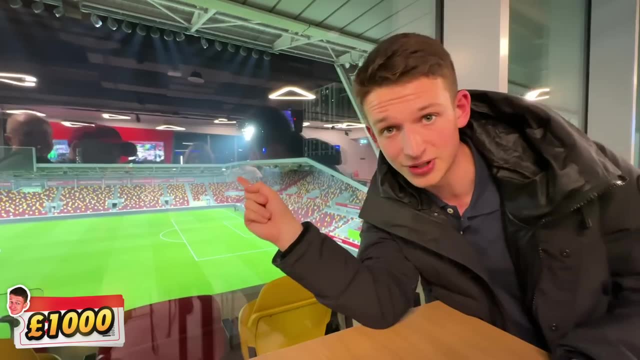 City Unbelievable. Why was he to not get that off the charity? The bar stays open an hour after a match so you can actually enjoy yourself and see them take away the goals. They've done a great job. The groundsmen credit to them. everything's gone already. 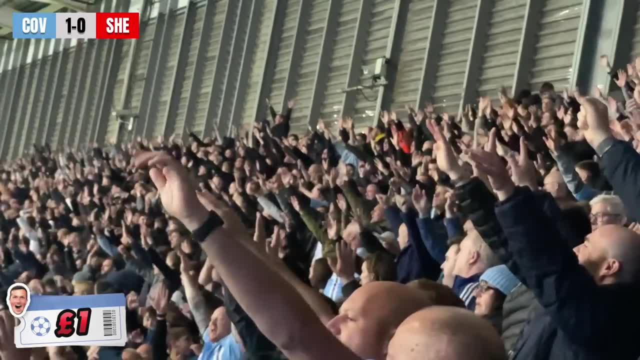 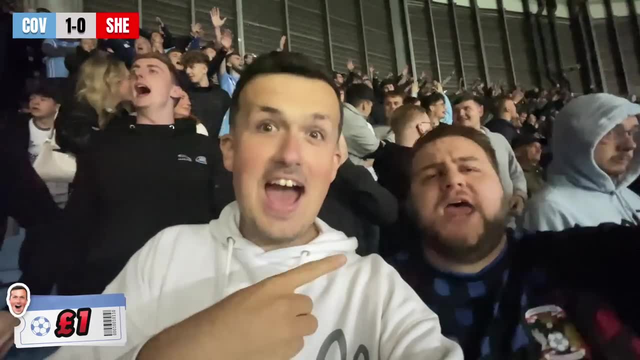 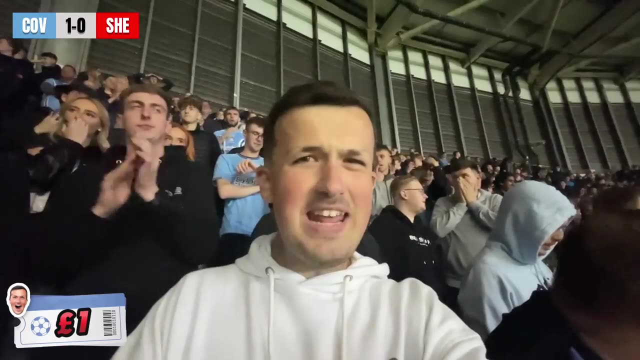 City, City, City, The best fans in the Championship. Yes, we are Exactly, Exactly. Get together, we will be the best. Stop the emotions, Get the atmosphere. West London derby- They've got to be prepared for this. 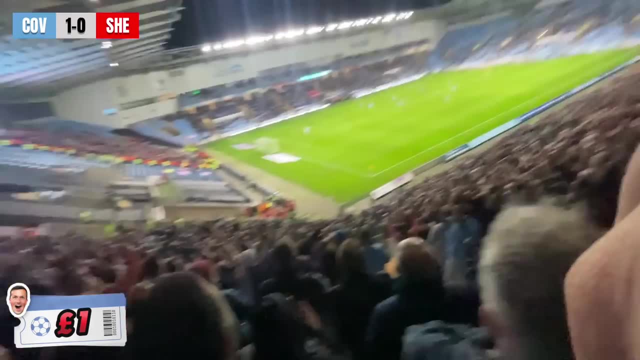 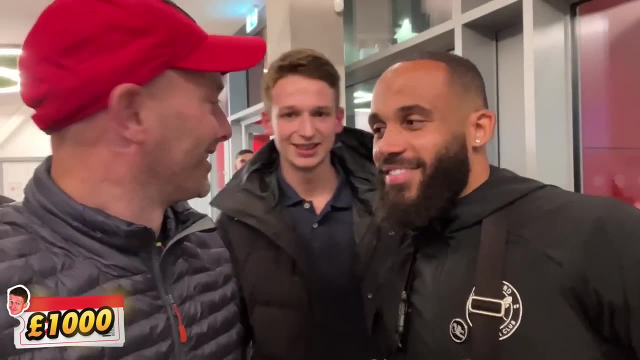 I'm telling you, Fionn And the Suns are in to get it. They've got to get it. They've got to get it. Wait a minute. that's Brian Mbwemo, the forward for Brentford. Yeah, 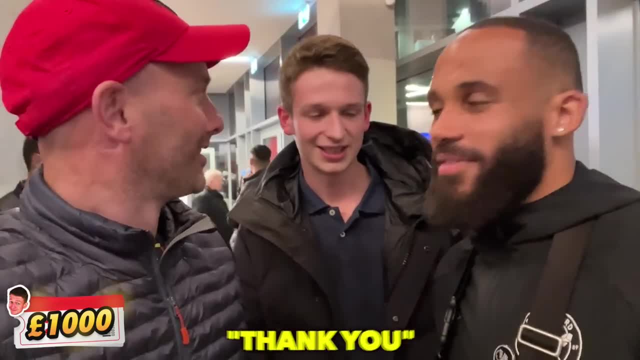 You've played so well for us. we're so happy man. Thank you so much. This £1 has been worth it, hasn't it? It's been worth it £50.. Fionn has not had as good a time as I have. 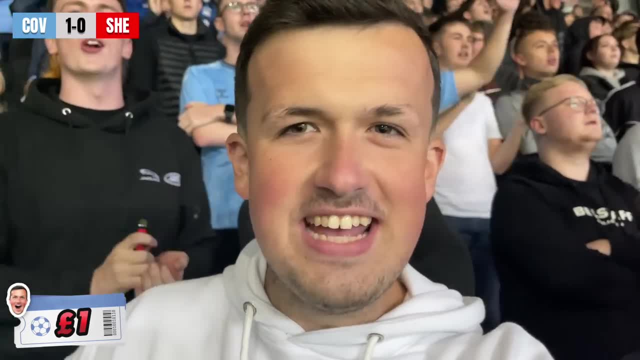 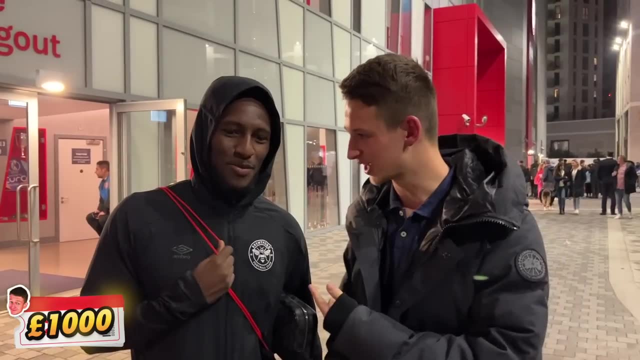 with the fancy atmosphere, with the limps, with the scenes, the last-minute goal, Fionn hasn't got that. West London, West London, There's Thogden speaking to Shandon Baptiste, the central midfield dynamo. 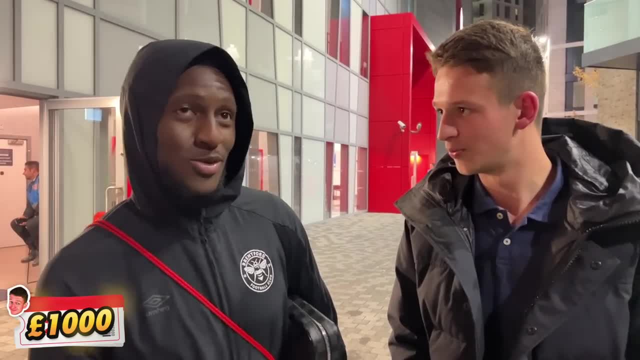 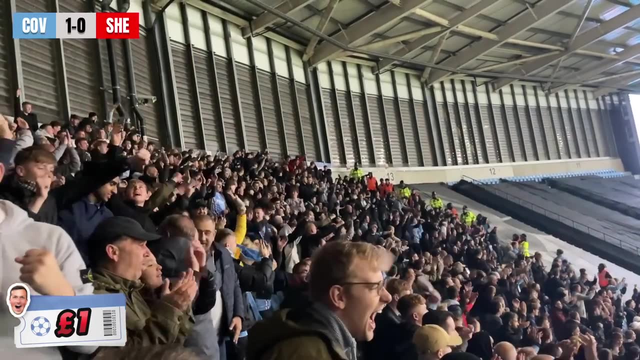 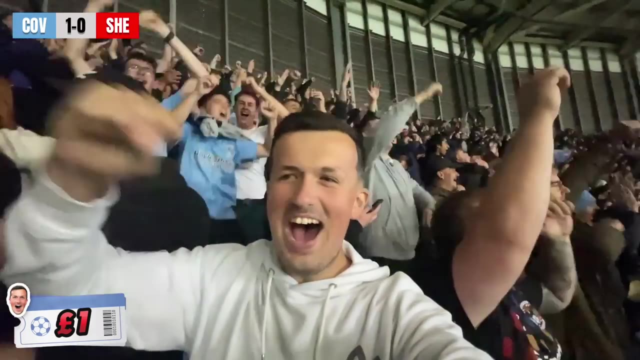 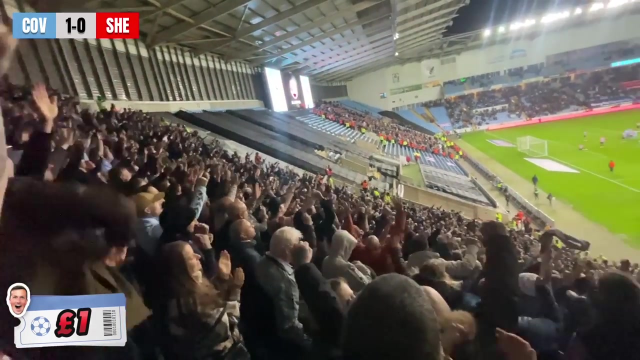 Good draw, Yeah, good draw. you know We're trying to get the three points, but they've got to win If we get 10,000 likes. I'm challenging Shandon to a little challenge. If the Commons have got to, let us know what they want. 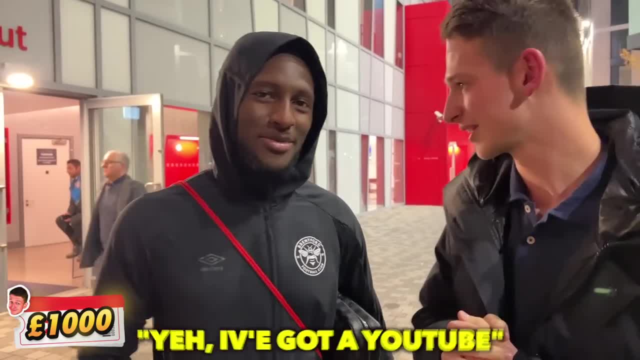 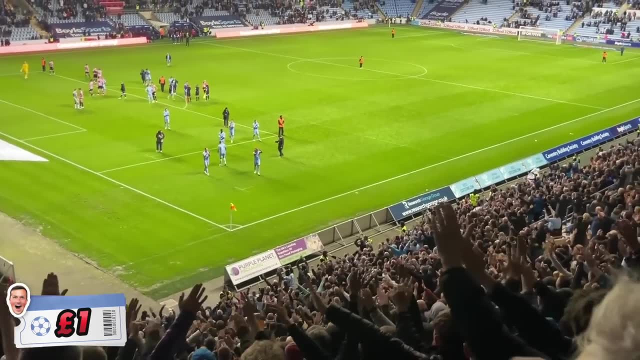 we'll make it happen. Should we make it happen? Shandon's got YouTube. Yeah, I've got YouTube as well. so Really, Yeah, Look at this, The passion for the fans. It doesn't compare to all the corporate money from your league.